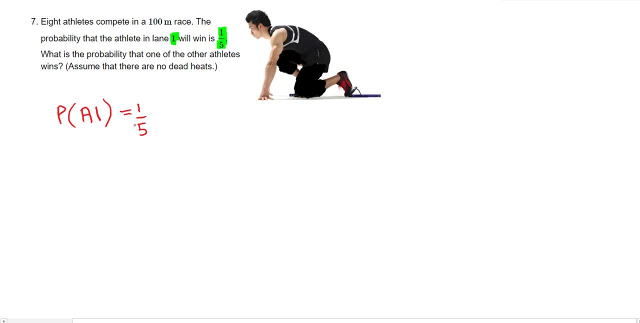 what is the probability that one of the other athletes wins? okay, so, not this athlete, but any of the others. so we know, the probability of athlete one plus the probability of athlete one not winning- and not is denoted by this little apostrophe sign- should be added together to give you one. okay, now what are the missing pieces? now, we don't know the. 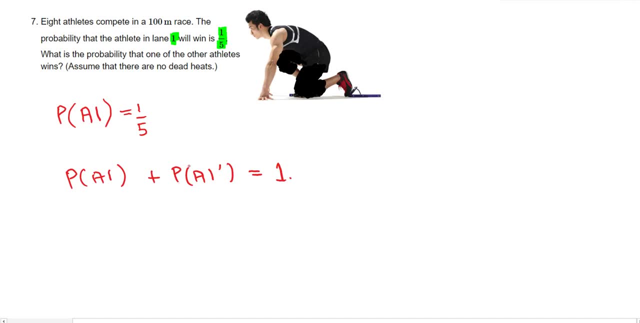 total probability of. we know the total probability but we don't know the probability of athlete one not winning. but however, we do know the probability of athlete one winning, so we'll just plug that in plus, probability of athlete one not winning equals to one. we'll make probability of athlete one not. 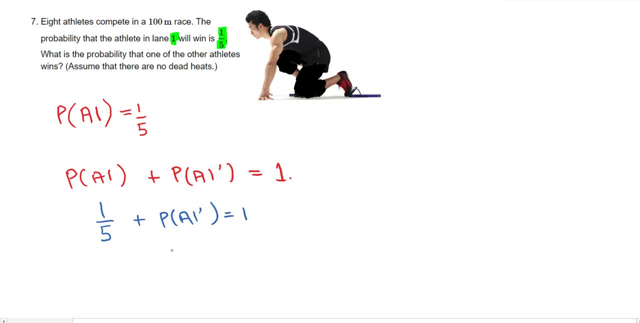 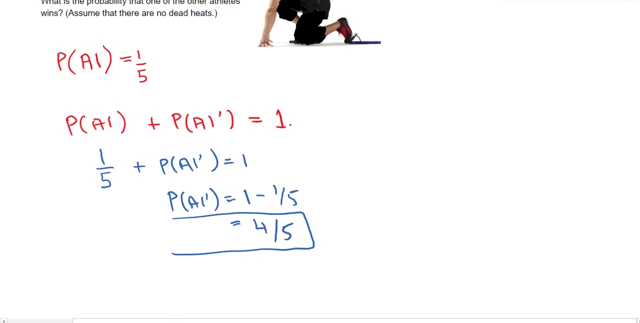 winning as a subject and move the 105 on the other side, you get the probability of a10 equals to 1 minus 1 over 5 and the answer to that is 4. so the probability that one of the other athletes wins is 4 over 5.. Okay, let's move on to another question. So the next question is: 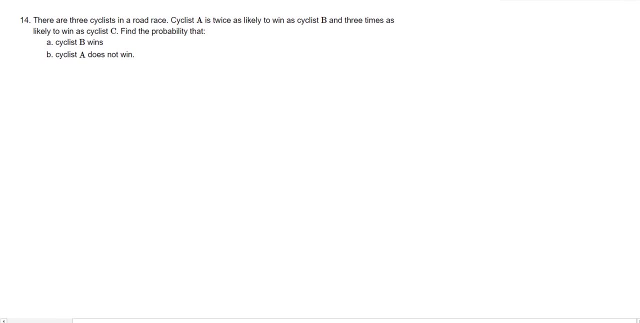 question 14.. There are three cyclists in a road race. Cyclist A is twice as likely to win as cyclist B. Alright, so I'm going to write these relationships down. So cyclist A: alright, so I'm going to just write that down as A. The probability of A is twice as 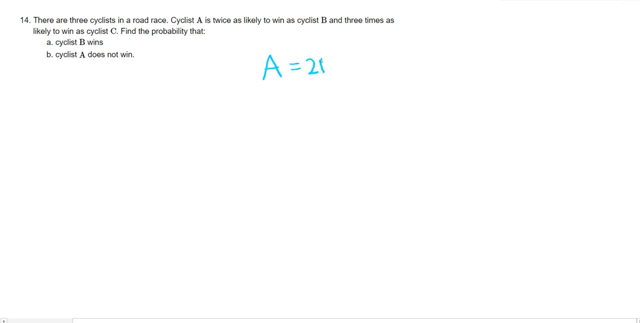 likely is equal to 2 times that of B. Okay, and that is this relationship over here. I'm going to choose a different color and we're going to continue reading the question. And so cyclist A is twice as likely to win as cyclist B, and 3 times. 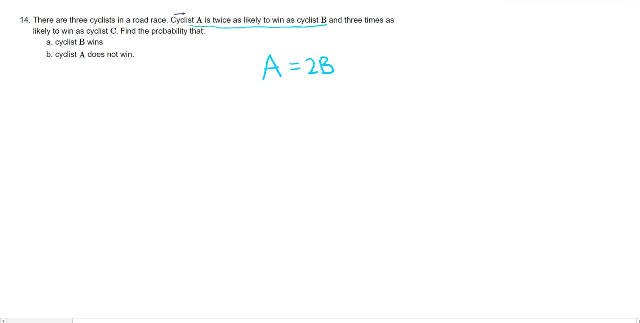 as likely to win as cyclist C. So again it's comparing cyclist A and saying that it's three times as likely to win as cyclist C. So A is also equals to three times C. Okay, now the question goes: cyclist B find the probability that 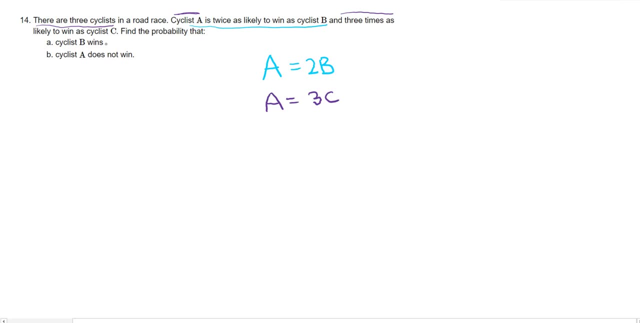 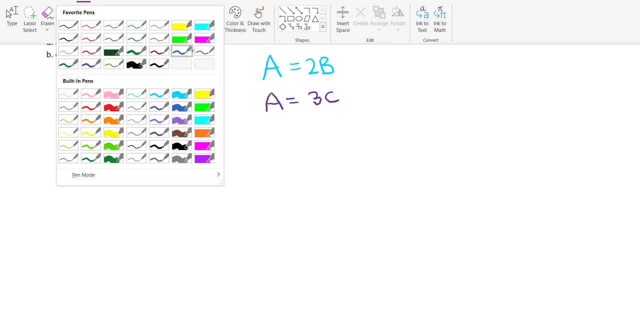 cyclist B wins. So we need to find what the probability of just B is, and for solving this, this is not as straightforward. what we're gonna do is make these equations that we have. So we have two equations: Equation 1, which is A. 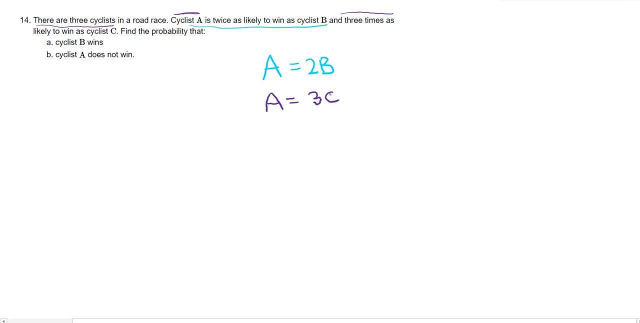 equals to 2B and the equation 2, which is A, equals to 3C. we're gonna make B and C the subject of this, Because we know the cyclist A has a probability of winning as A, but what's the probability of B winning? 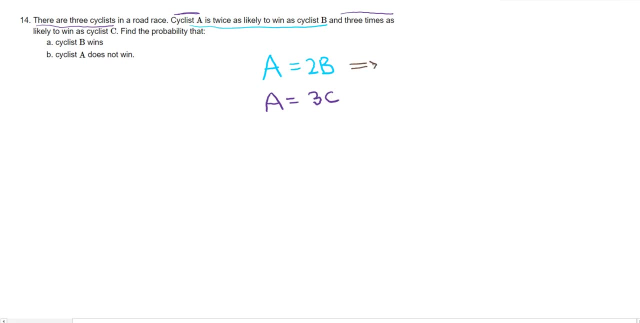 so that will be if I simplify this and make b the subject and just literally divide two on both sides. on that I get b equals two. I can just write a equals two equals to b, a over two equals to b, sorry. and in the second one. so that is my equation for b and for my second one, let me 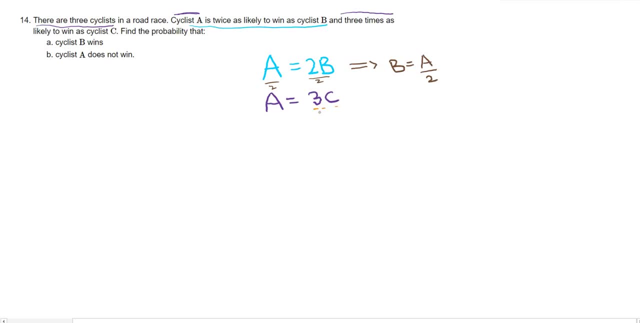 color. it's just going to be literally dividing by three on both sides and getting rid of three with the c, so I make c the subject. c equals to a over three. all right now it would make a bit more sense as to why we did that in the next step. the next step is: we know the total of all. 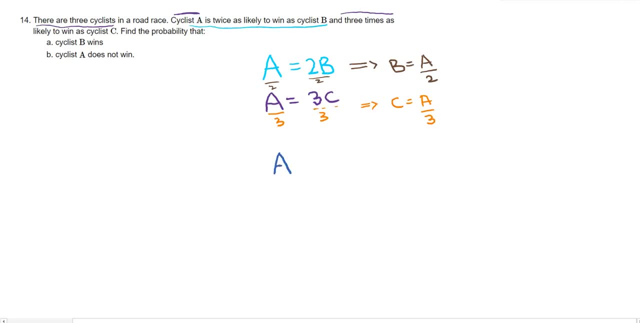 probabilities added together would always equals to one. so a probability of a plus the probability of b plus the probability of c: if I add them together, I should get a one. okay, so the probability of a: we don't know what it is, but we know that it's denoted by a. and if you look at b now, we have a relationship of b, which 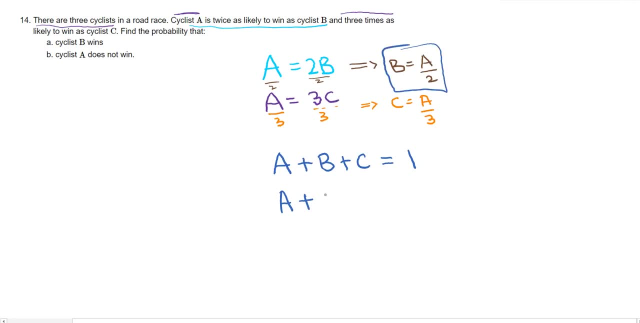 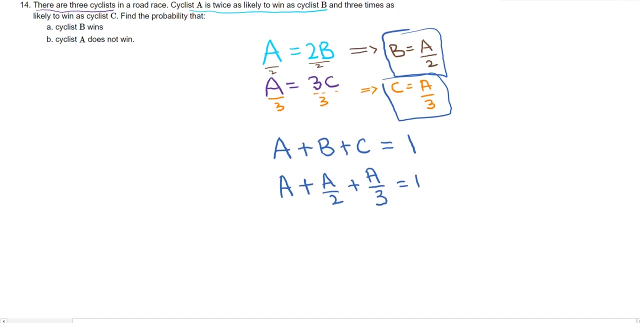 is in terms of a, and I can just use that. so b is equals to a over two. I'm just going to put that there: a over two. and then for c- I have a relationship with c as well- in terms of a, and which is: a over three equals to one. all right, 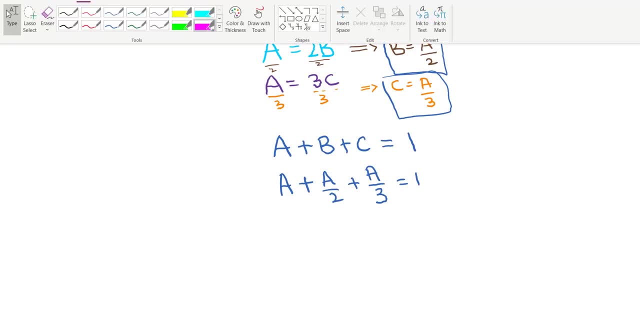 when you add this fraction towards the left side of the equals to sign, you realize that you end up with. so if you just a brief, you know- recap of how to do how to add fractions, you need to have the denominators exactly the same, so the lowest common denominator, or LCM. 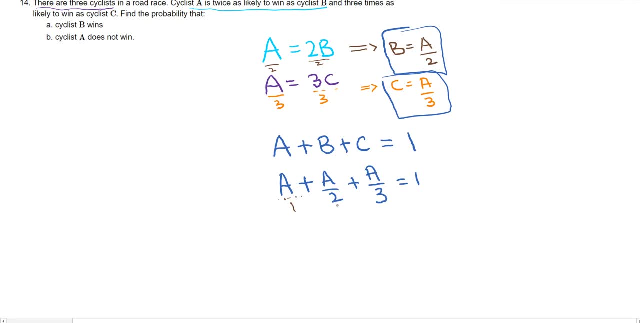 lowest common multiple of these three numbers- one, two, three- is going to be six. all right, so if you list down the table of one, table of two, table of three, where do they meet up? the first where they all meet is six. all right, so they. so I need to have the denominators of six on both. on. 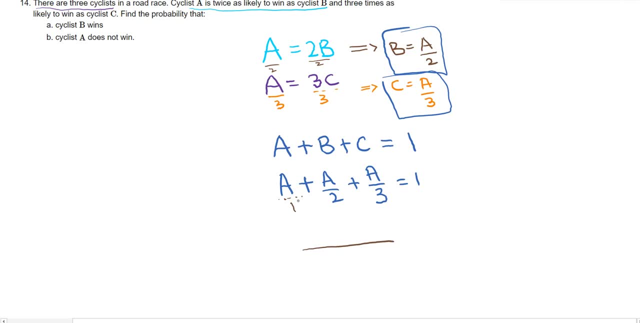 all on all these fractions. so if I want to get this to become a six, I need to multiply the above one with the six as well, and this one I need to multiply by three, so I'll multiply that by three as well, and this one I need to multiply by two, so I can get that two, two as well. all right, so if 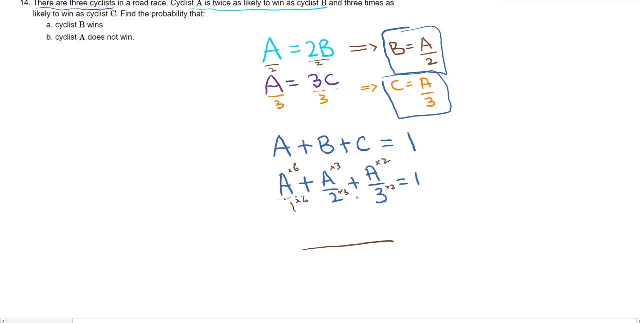 you notice the denominators are now all sixes. all right, by multiplying those. now, whenever you multiply something in the denominator at the same number, you multiply it by two and you get the should be multiplied in the numerator as well. so i've got 6a plus 3a plus 2a and it's divided by 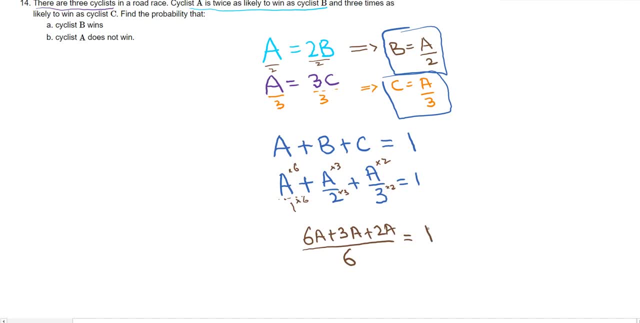 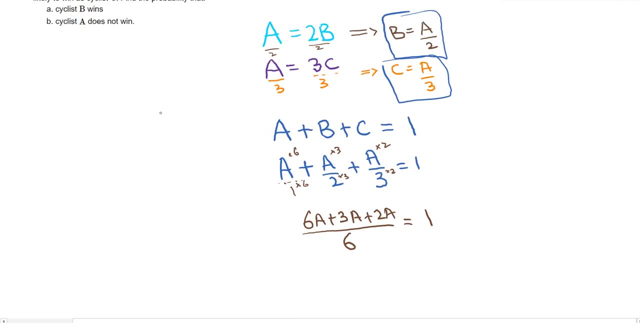 the whole thing divided by 6 equals to 1.. all right now, this is where algebra skills will come in handy, and we need to move that 6 now from the denominator to the numerator, to the other side. now the way to get rid of something which is in division: you multiply it. so i multiply. 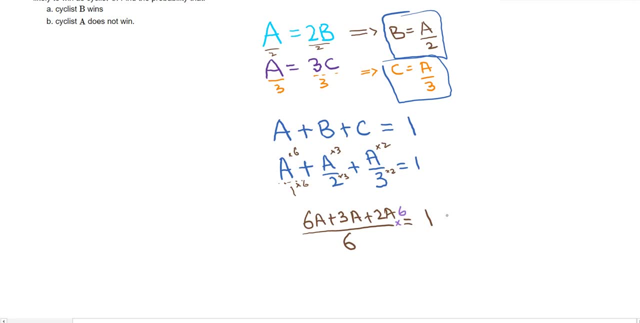 uh, this over here by 6, okay, and i multiply on the other side by 6 as well. so this times 6 and this divide 6, cancels out or become 1, and i only end up with: uh, now i'm remaining behind with 6a plus 3a plus 2a, that's 11a. 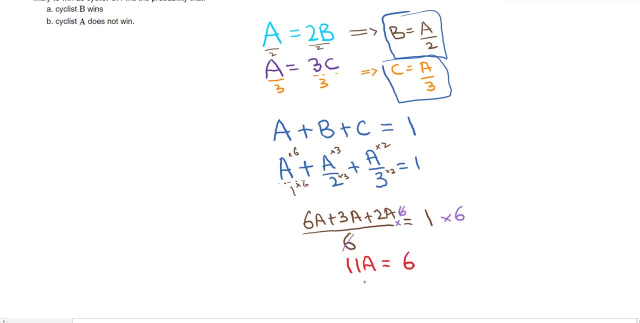 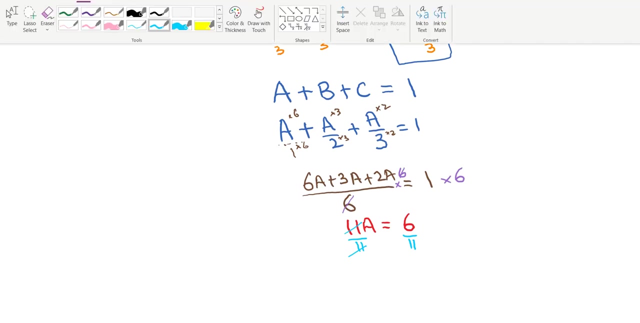 equals to 1 times 6 is 6. okay, and now a simple division on both sides would just give me a value of a. so divided by 11, divided by 11.. okay, and let's divide. just gets rid of that. it becomes 1. 11 divided by 11 is 1 and ta-da, my final answer is a equals to 6 over 11.. 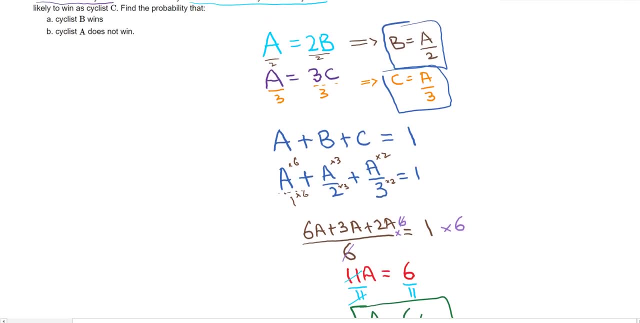 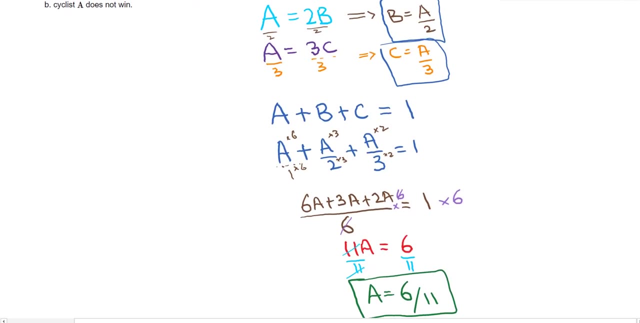 all right, we found the answer happy? i don't think so. let's go back. the question says: find the probability the cyclist b wins. it wasn't even asking us for a, but now we have one missing piece of the puzzle already found. now it's much easier. 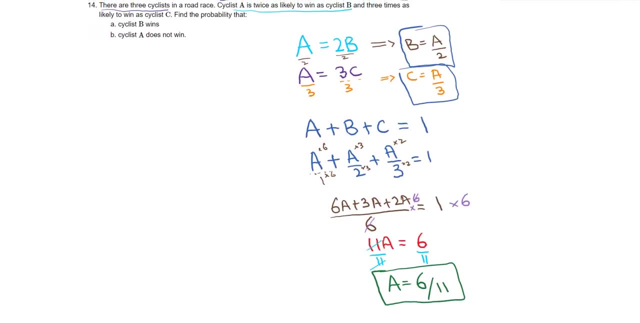 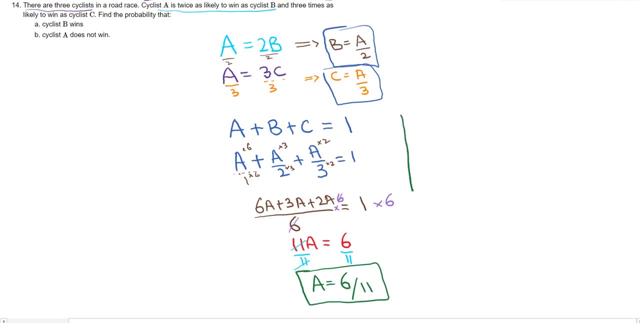 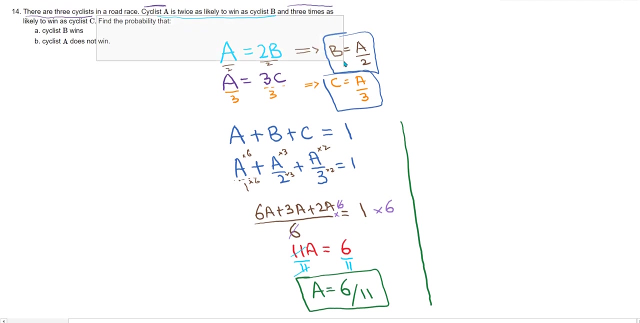 for us. let me zoom out a little bit. sorry, it's too zoomed out. we zoom in back, zoom back in. all right, i'll do the working out for b, b and c. i'm much, much simpler because we already have an equation set up for them, all right. so if you remember, we had, uh, this value for b over here, b. 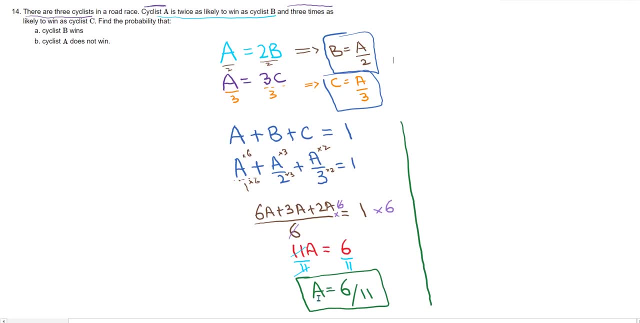 was equals to a over two, and now what we'll have here is the polynomial. so we settled out the two, and now we know what a is all right. so all I'm gonna do is just sub my a into that all right, and let's see what happens. so if my B is equals to a over 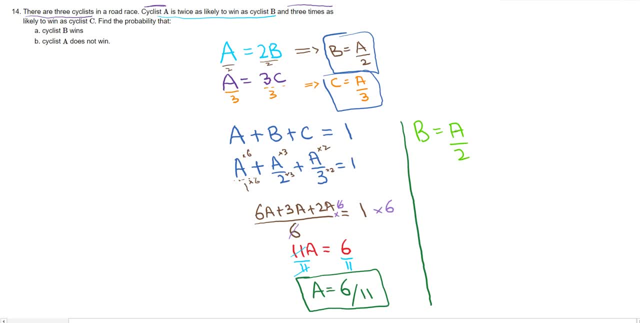 2 and a is 6 over 11. it's gonna sum that in: so B equals 2, 6 over 11 and this over 2. now let me rewrite this so it's very clear as to what we are doing, otherwise it will be confusing. so 6 over 11. I'm gonna write it like this, and this whole 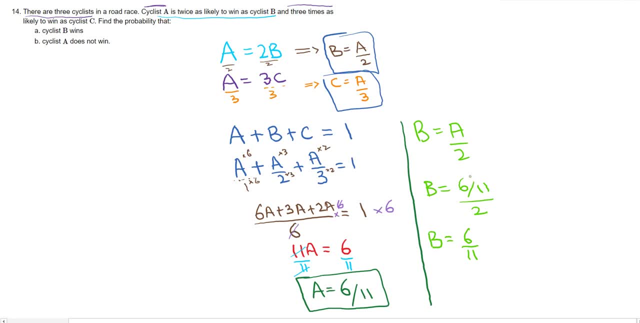 thing which is a binculum sign. all right, there are two binculum signs here, minus 6 over 11, then the whole thing over 2, so that over 2 is like a divide by 2. now, remember, over means divide, okay, so it's divided by 2 now in primary, you might. 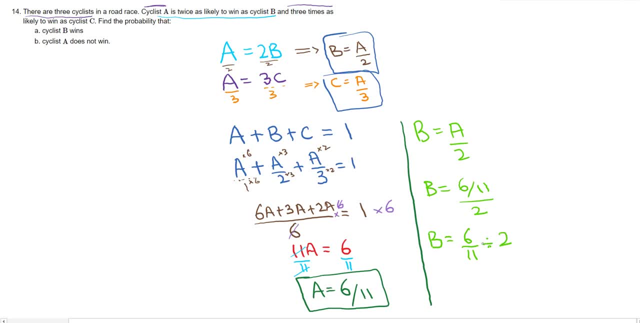 remember, whenever you have questions like this with the divide sign, what do you do? you do the reciprocal by changing the dividing formula: multiply so that will become 6 over 11 times 1 over 2. okay, and when you multiply this fraction together and simplify it, you will get your answer as: 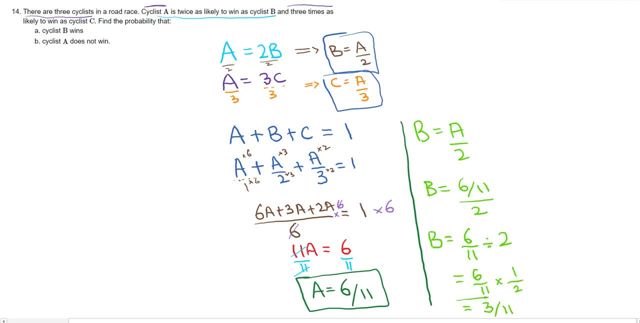 3 over 11. okay, that's your answer for a. this is part a answer. now, while we edit, let's go ahead and find C as well. okay, because that's going to be used in time. B now see the relationship of C. was that a divided by 3? all that? 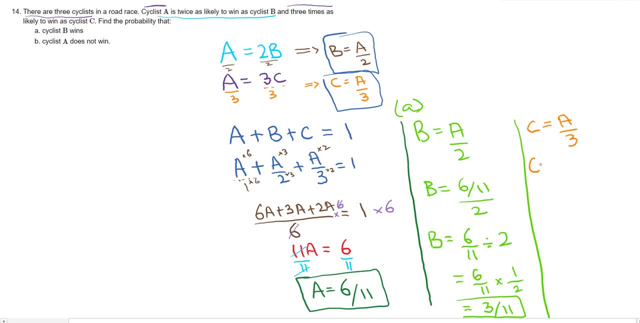 now a is 6 over 11. already found it, so I'm going to sub that value in same rule: 6 over 11, divided by 3, and I'm going to rewrite this in a way that we can understand easily as to what's going on. divided by 3 and the same rule again: do. 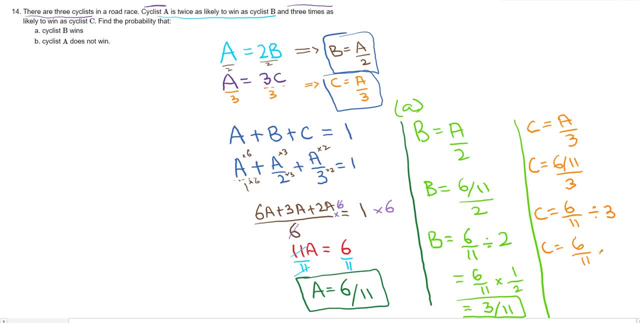 the reciprocal, you get 6 over 11 times 1 over 3 and guess what you end up with? you end up with 2 over 11. and these are answers for a, B and C. now let's read part B. and part B says: cyclist a does not win. now 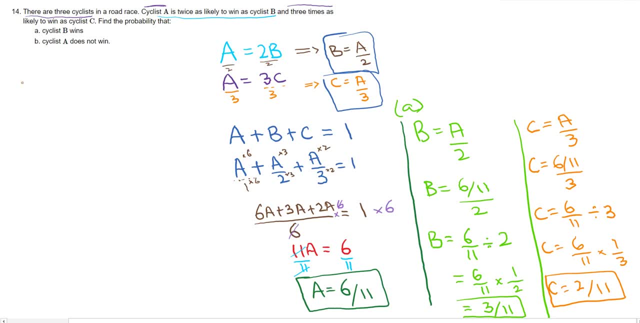 remember, does not win. okay, it does not win, so I'll do B here. let me change the color. it seems so. part B says probability of a not winning. okay, now if you know the probability of a, we can just find the a not. a not is going to be, because we know the probability of. 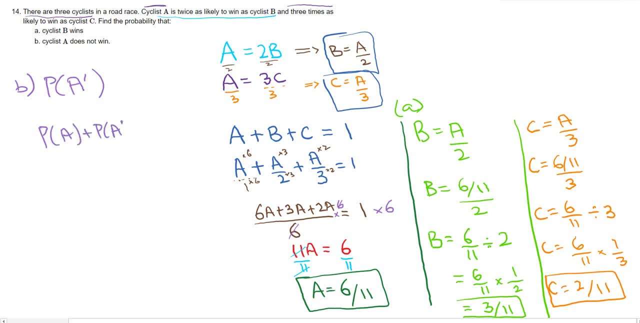 a plus, probability of a not is going to equals to 1. okay, so probability of a was 6 over 11. how much is probability of a not going to be? to make it a 1. okay, what is it going to be? question mark is 2- 1. now what we're doing it is that you move this 6 over 11. 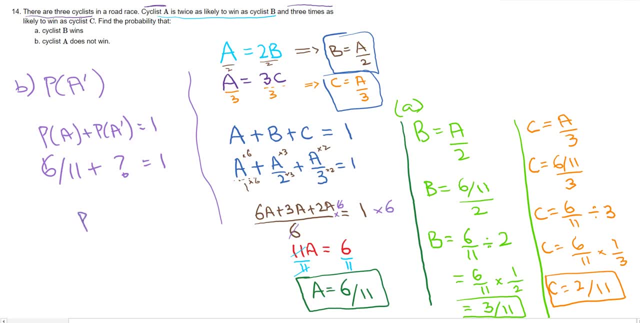 on the other side. okay, and you find that probability of a not is 5 over 11. okay, or the other way of doing it is: you go to part, you go to your parts over here where we found the probability of B and C, you add these together. okay, because a. 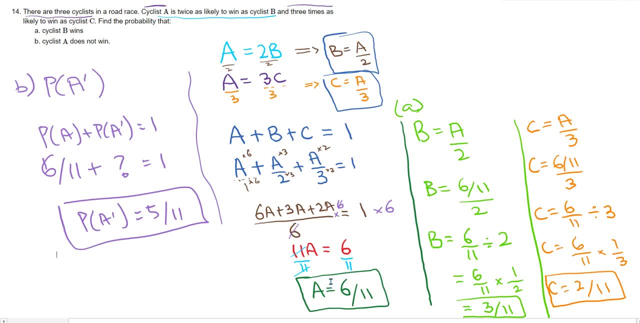 not meaning either B or C, because there's only three races, like it's told in the question. so it's either a, B or C. if a doesn't win, then either B will win or C will win. so 3 over 11 plus 2 over 11 and you get the. 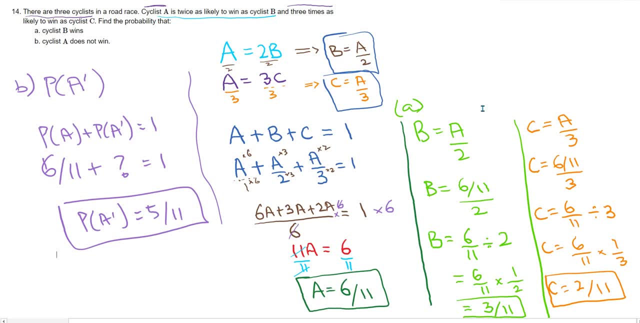 same answer: 5 over 11. okay, hope that makes it clear. inshallah, all right. Jazakallah Khair, until I see you in the next video.